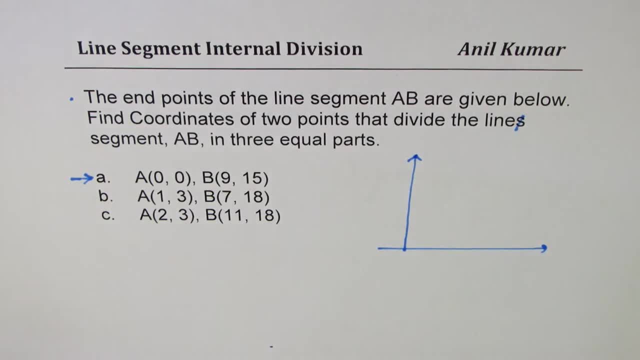 So let's say that is XY plane. Point A is at the origin. So let me make a line, segment AB And let's say that point A is at the origin. So let's say that point A is at the origin. And let's say that point A is at the origin. 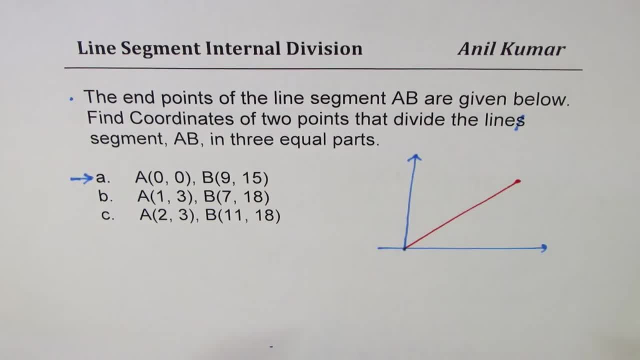 So let's make a figure kind of like this, where we have point A at the origin, which is 0, 0.. So A and B are these two points. B is 9, 15.. And A is 0, 0.. 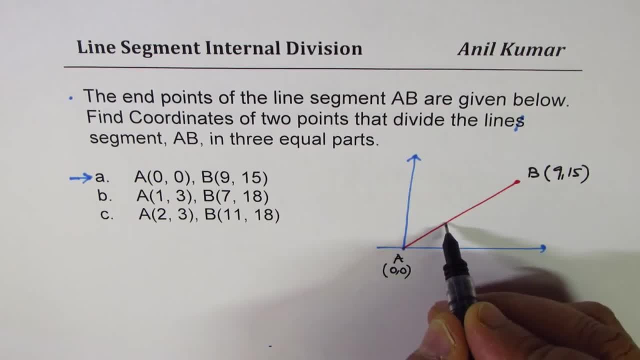 So we are looking for two points, let's say P and Q, which divide this into three equal parts. Let's call this point as P and this point as Q. The idea is to find X and Y values of these points, The concept which I am going to discuss. I'll solve this question without any formula. 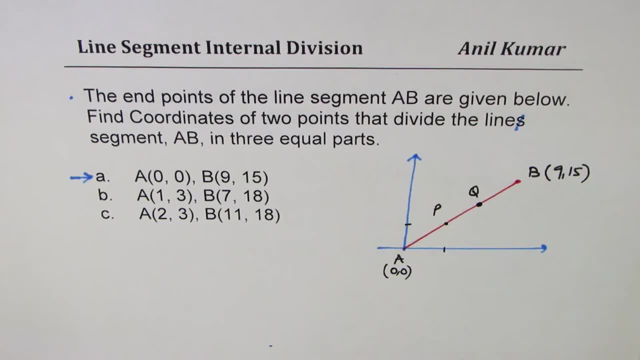 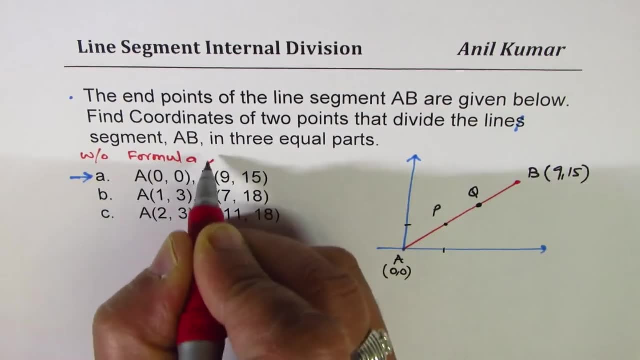 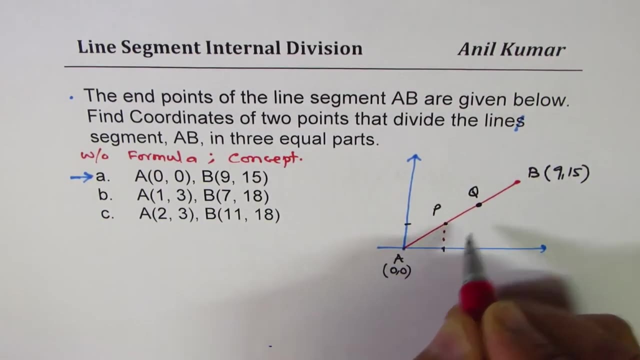 using a concept. So we'll do without formula. We'll do without formula. We'll use a concept. So we're just saying that let's divide it to three equal parts. That really means that these parts are equal, And vertically we have the situation where these parts are also equal, right? 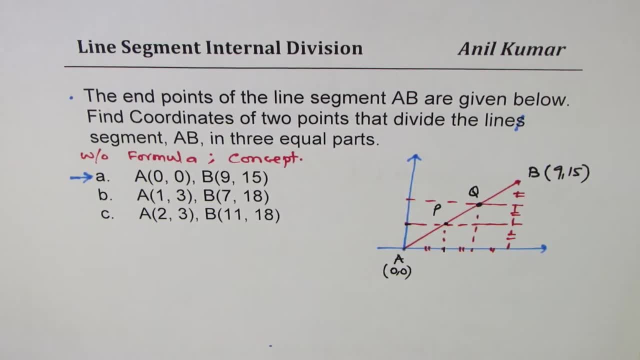 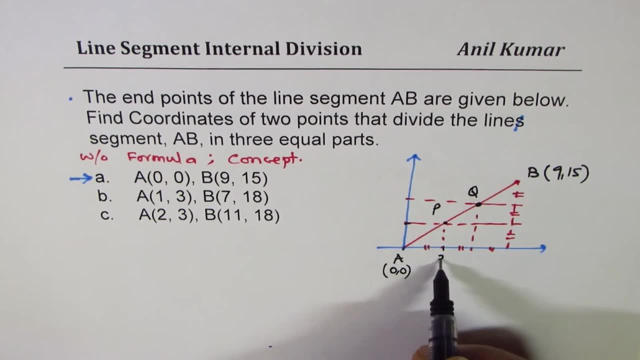 So, logically, what can you see? Clearly, total length from here to here along the X axis is 9, right So? So each is 3,, 3,, 6, and 9,, three equal parts. The Y values: we want to go up to 15.. 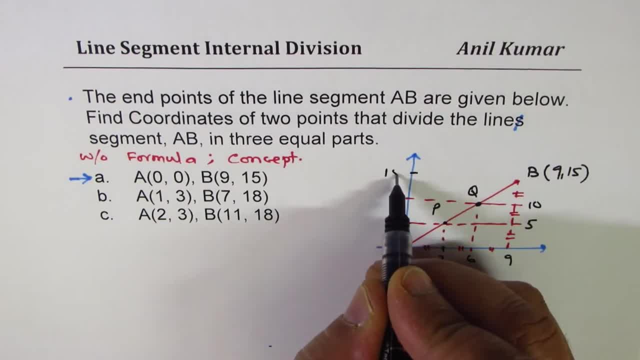 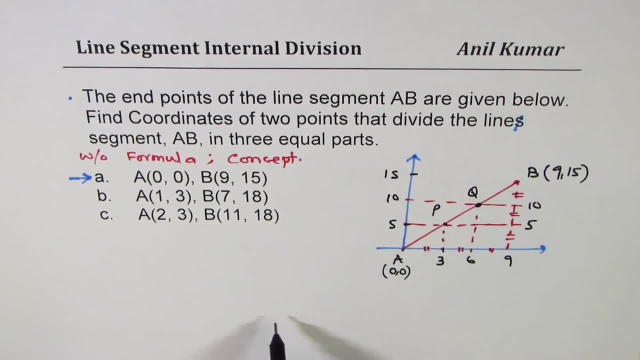 So it could be 5,, 10, and 15, right? So that gives you the coordinate points of P, Q and R. So we have point P as 3,, 5.. Point Q as 6, and 10 as our answer. 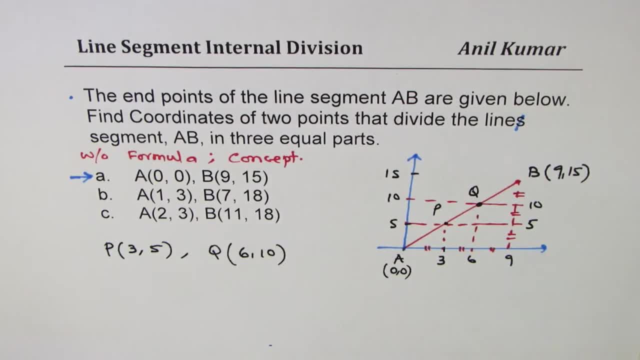 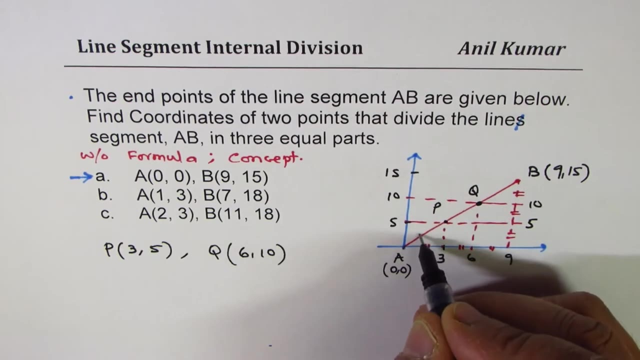 Does it make sense to you? Perfect, So that is how we are going to do it. Correct, That is how we are going to do it. So we get now points P and Q, which will divide the segment AB into three equal parts. 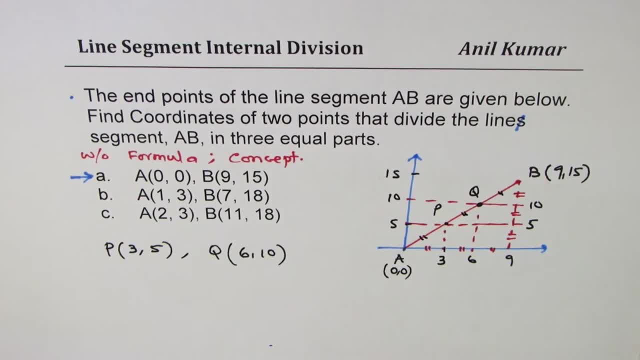 So that becomes our answer. Do you see how we got it right? So basically we are saying If there are two points, endpoints are A and B, then the formula is kind of X2 minus X1 divided by 3, and Y2 minus Y1 divided by 3. for the point P: 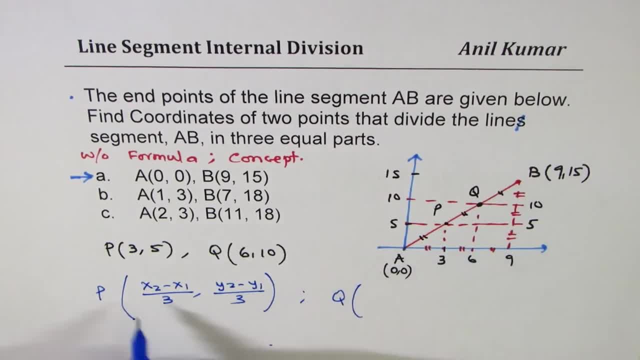 And for point Q, since it is two-thirds. so we'll say 2 over 3 times X2 minus X1, and Y coordinate is 2 over 3 times Y2 minus Y1.. Does it make sense? Perfect, So the total length has been divided to three equal parts. 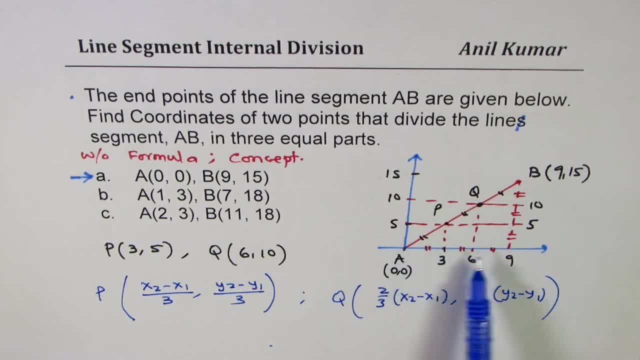 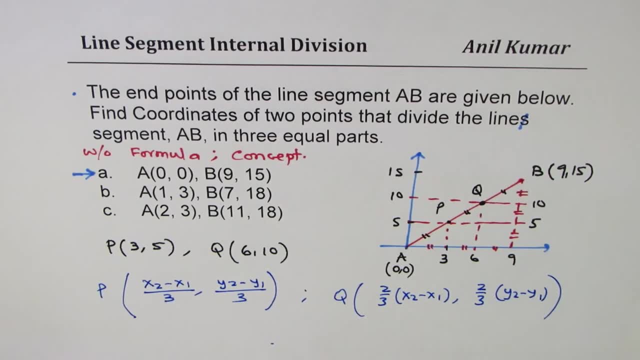 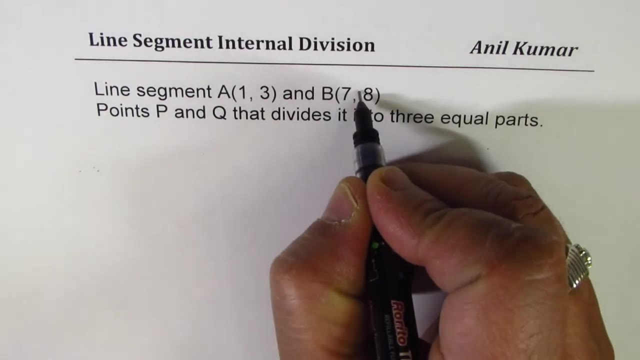 P is one unit of A and Q is two-thirds of the units of A. right, So you get your answer Perfect. Now let's take the second one Where there is slight difference. Well, here is a typing error. It is 18, not A. 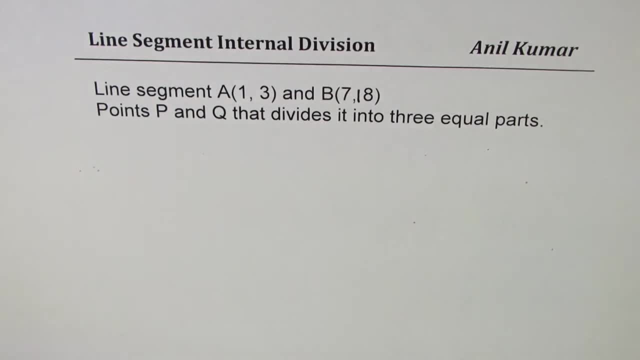 It is 18, not A. Okay, So now we have a line segment. This time the line segment has been translated towards the right a bit, So let me redraw this. We are saying AB, but A is not at the origin. 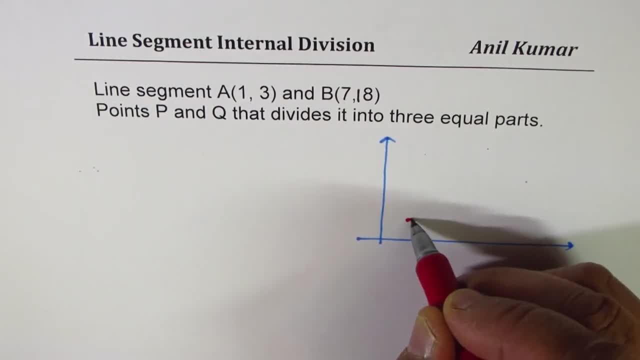 It is at 1, 3.. So we say, let's say this is A and this is B. right, They are not to the scale. We are trying to understand the concept. Is that okay? Okay, And we'll follow the same. 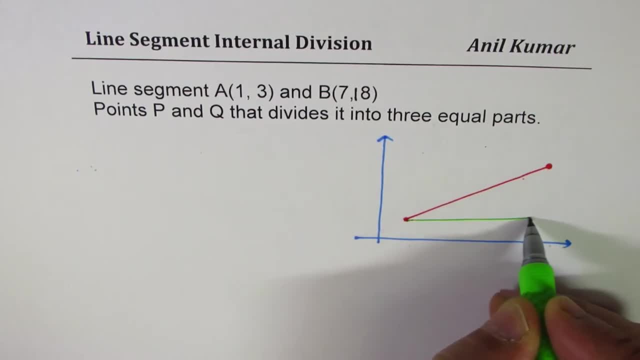 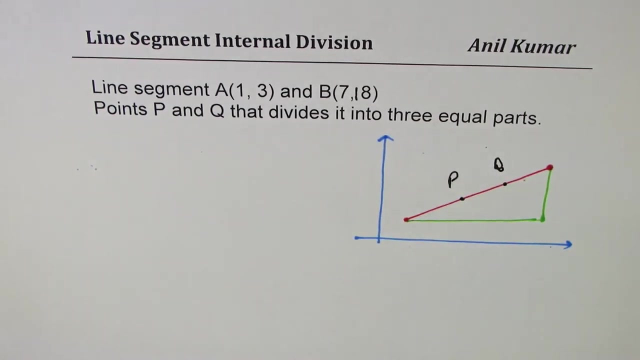 Same thing which we did last time. This time the triangle is kind of here. Now we want to divide again, using two points, P and Q into three equal parts. That really means that we have to divide this distance between A and B in three portions. 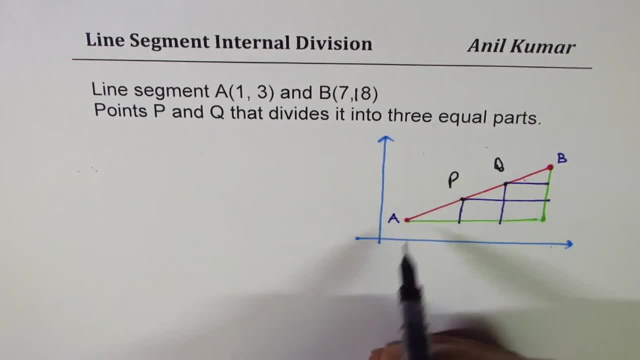 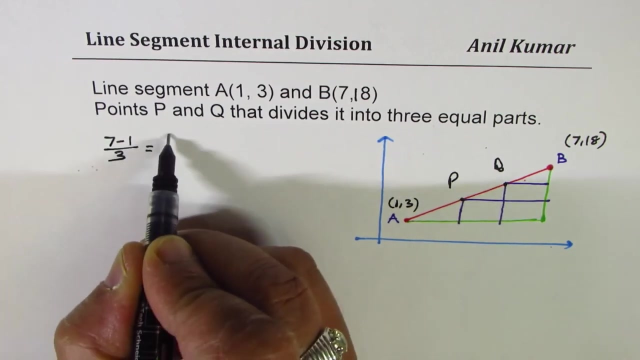 Correct. Now. A is 1, 3, and B is 7, 18.. So each unit is how much? 7 minus 1 divided by 3 is 6 over 3,, which is 2.. So from A we got 2, 2 units. 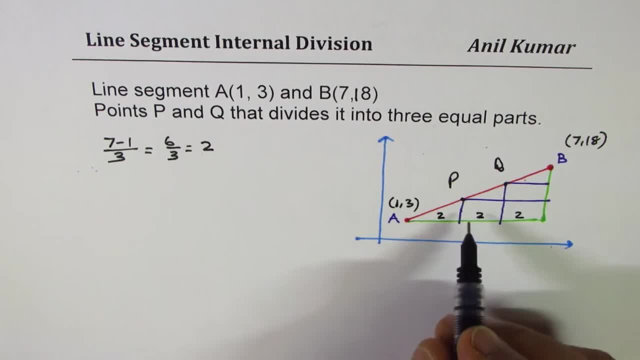 Do you see that? 2 units to the right. So that means the X values. here are what The X values will be. initially it is 1, right. This point here is at 1.. So what is 1 plus 2?? 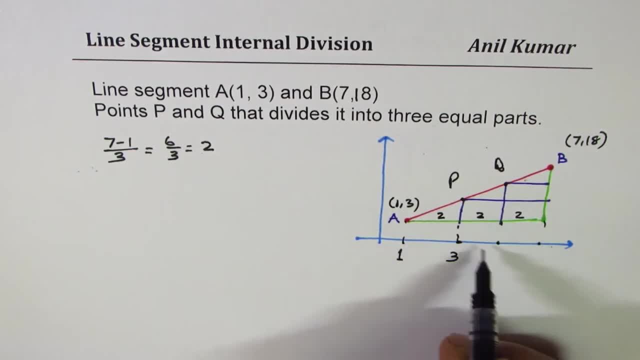 It is 3.. And what is 1 plus 4?? 2 more 5. And 2 more gives you 7.. That makes sense, Is that true? Now let's look into the Y values. Y value is 18.. 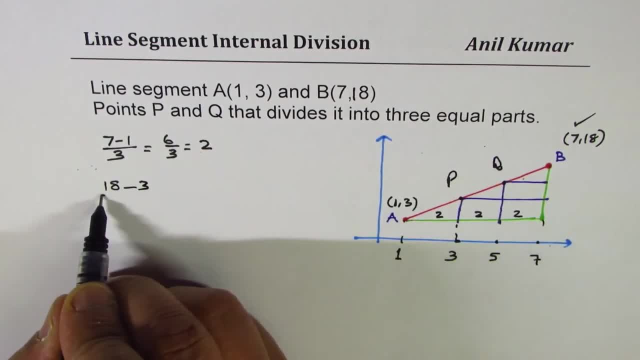 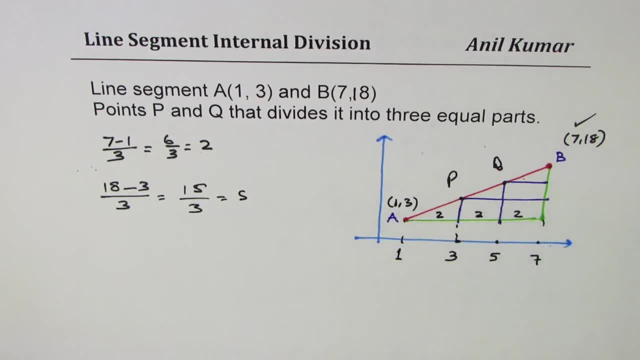 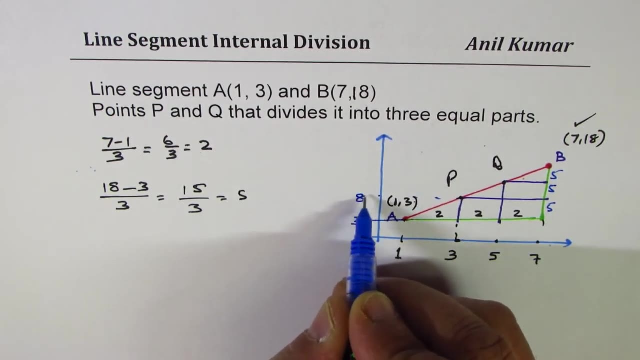 So it is 18 minus 3 divided by 3., Which is 5.. So each unit is 5 above right. So this is 5, 5, and 5 above this point, 3, right. So from 3, if you go 5 above 5 plus 3 is 8.. 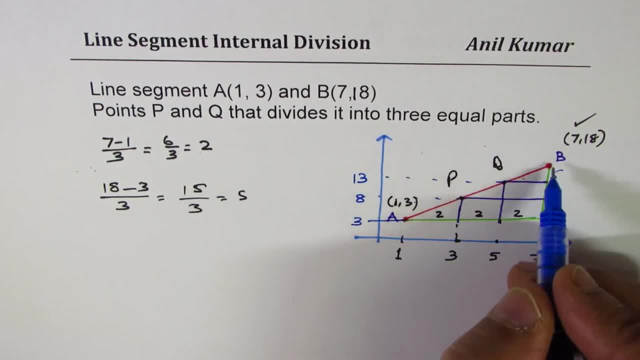 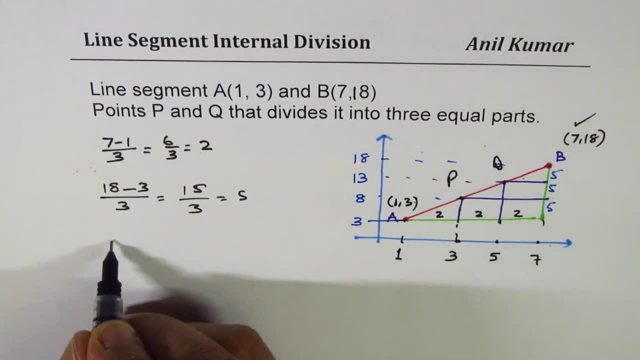 And another 5 will 13.. And next 5 will take you to 18.. That makes sense. So you get your answer right. So you get point P As this coordinate 3, 8. And Q as that coordinate 5, 13.. 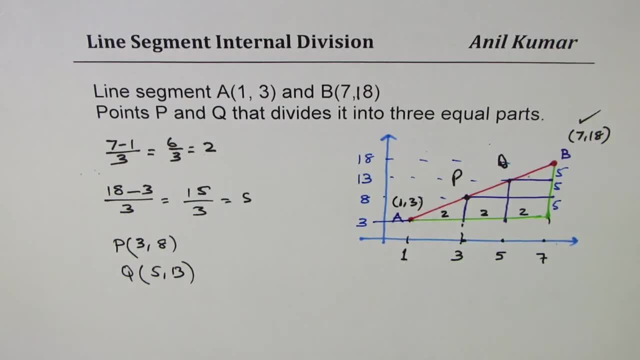 So I hope with this you understand the concept. So the idea is, if you are dividing into three equal parts, we could see those parts being divided along X axis and along Y axis, Right, So we can add each portion to the initial value A. 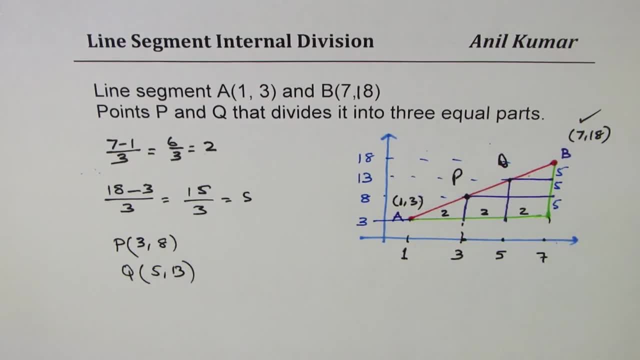 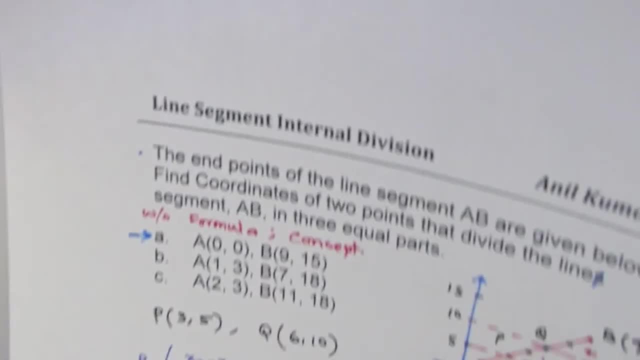 To get our answer. Is that clear? That's how we're going to do it right, So I'll leave the third part with you, which is So question number 1C. The point A is 2, 3, and B is 11, 18.. 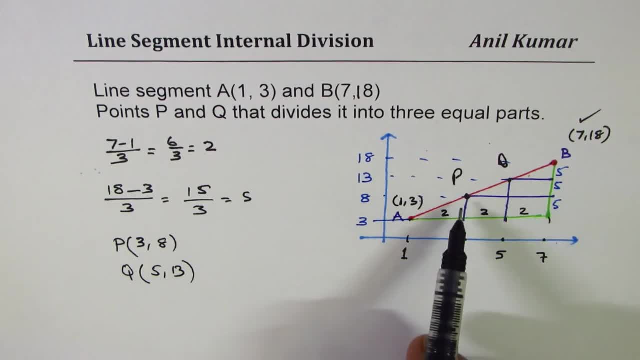 So let this be a question for you, right? So we got the answer here. Now for you, try this out: Where point A is 2, 3. And B is 11, 18.. So I hope you should not have any difficulty in solving this. 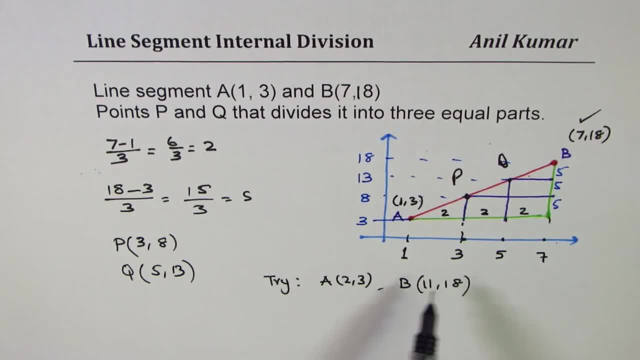 So 11 minus 2 is 9.. Divide by 3 is 3 units. Add 3 to 2 to get the first point. Y values: 18 minus 3 is 15.. Divide by 3 is again 5.. 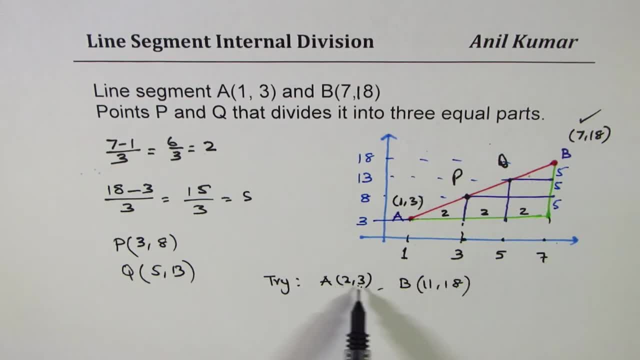 So you can again keep on adding 5 to A values- initial value. Is that okay? That should give you the answer. So I hope the concept is clear. Feel free to write your comments and share your views And, if you like, and subscribe to my videos, that would be great. Thanks a lot for watching. 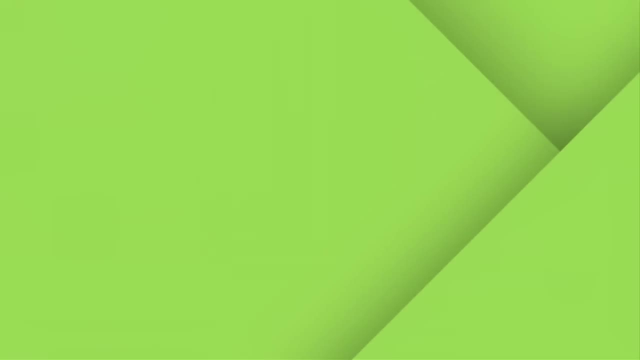 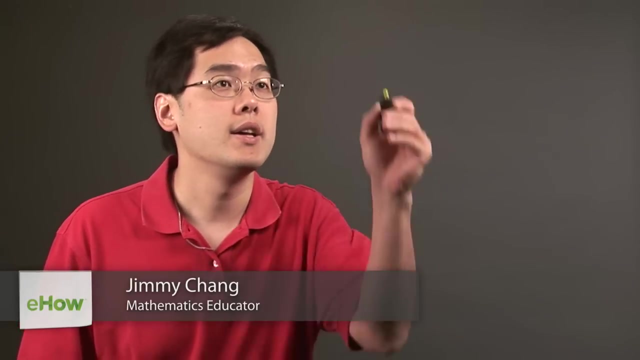 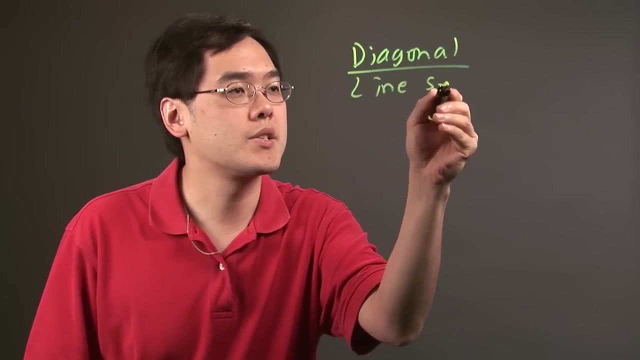 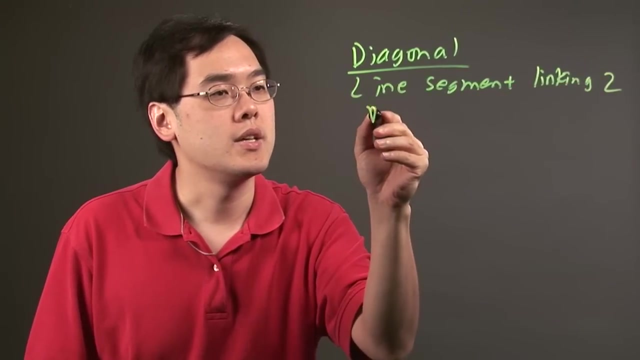 Hi, I'm Jimmy Chang. We're here to talk about what does diagonal mean in math? Now, diagonal is used in geometry, where diagonal is a line segment that links two vertices. But the important thing to think about is that the vertices have to be non-adjacent, In other words, they 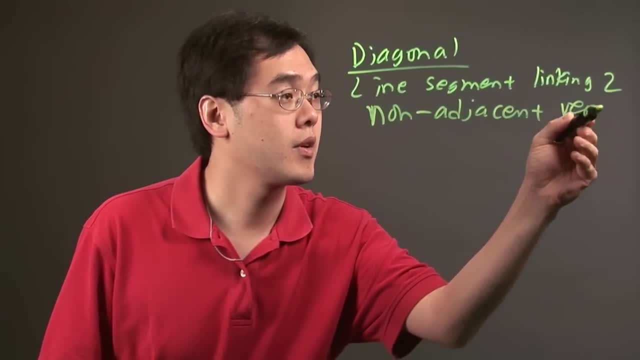 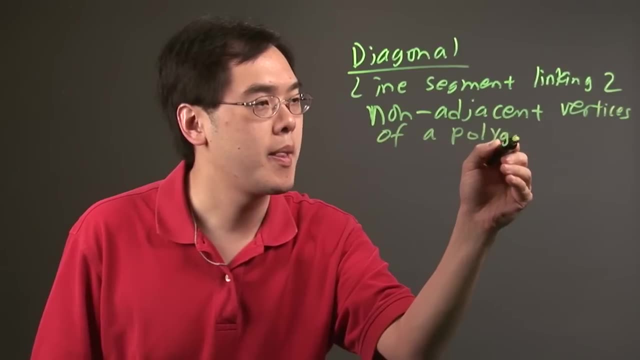 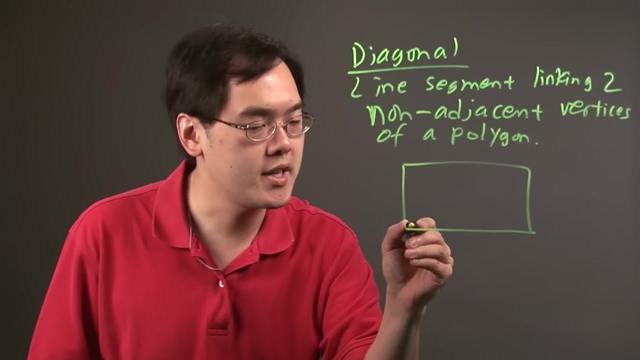 cannot be next to each other And it happens in a polygon. So it's a line segment linking two non-adjacent vertices of a polygon. So if you have a rectangle, for example, you want to take into account that this, you want to draw a line segment from this vertex to 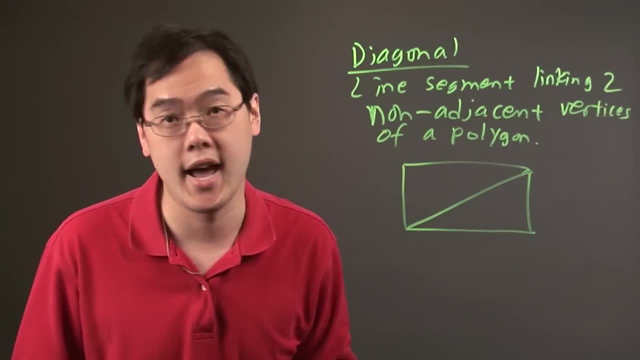 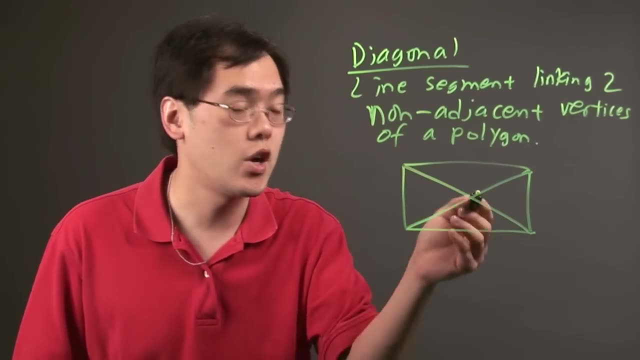 this vertex. Now, remember, the vertices cannot be next to each other, so this will qualify as a diagonal. Is that the only one? No, of course not, because if you have this, you have a diagonal drawn. This also qualifies because this line, to this line, joins two non-adjacent 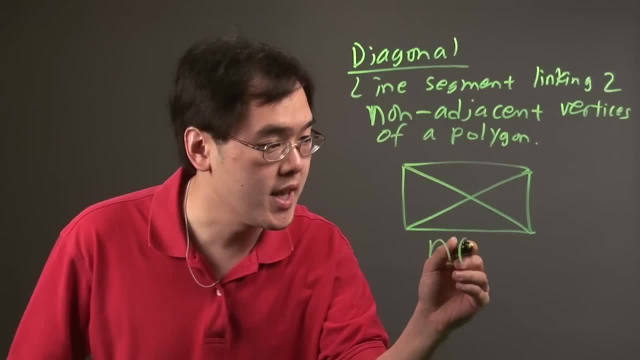 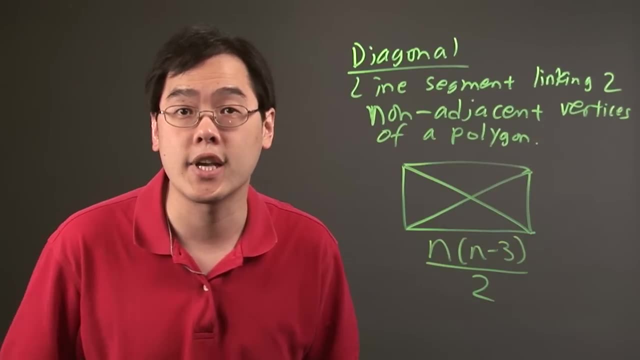 vertices. Now there is a formula associated with this and that is n times n minus 3 over 2, where n is the number of sides in a polygon. So to find out how many diagonals that can be drawn within a polygon, use this formula. So I'm Jimmy Chang and that's what does diagonal. 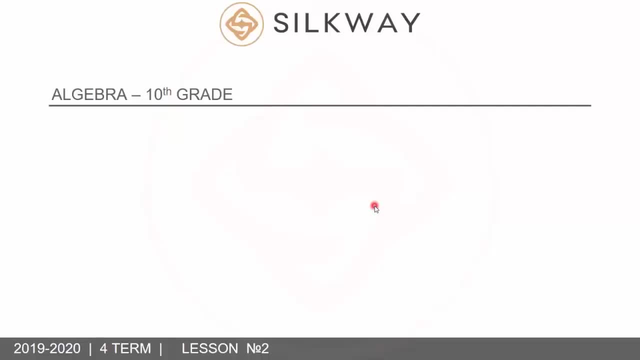 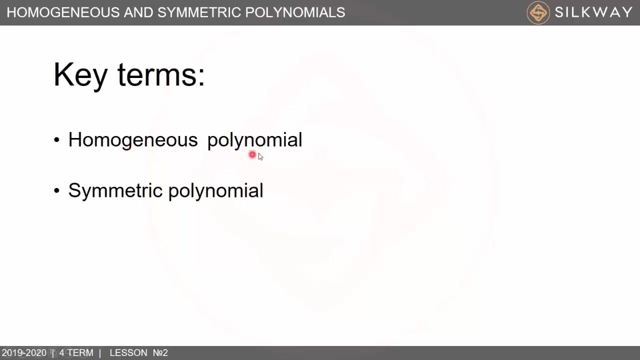 Okay, guys, welcome to our math lesson, and today's topic is homogeneous and symmetric polynomials. You will be able to recognize homogeneous and symmetric polynomials. Key terms: homogeneous polynomial and symmetric polynomial. Okay, write these terms please. And then, what is homogeneous polynomial?